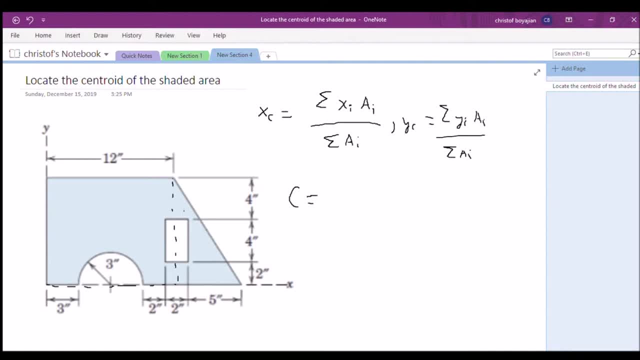 and now we have to make sure, whatever areas are shaded, we add those together and then the areas that are open, that have no shade, we subtract them. So here I'm going to label these as 1.. This rectangle I'm labeling as 1.. 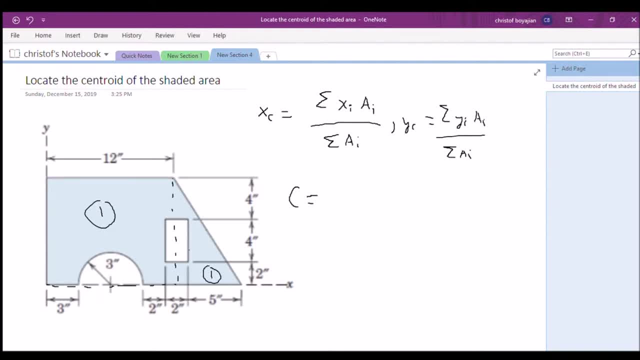 I'm going to label this total triangle as 2, and I wrote 1 in there. It's going to be 2, and then this semi-circle I'll say as 3, and then this rectangle right here is 4.. So I'm going to go ahead and draw these shapes. 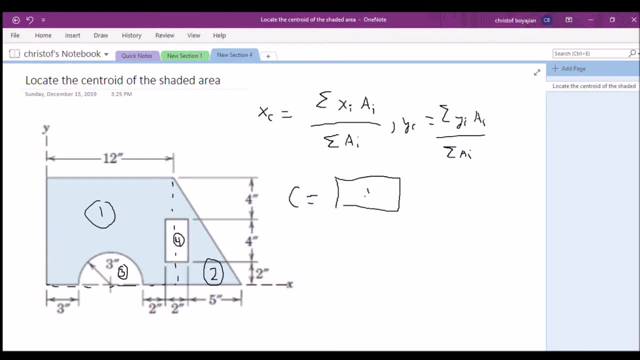 So centroid is going to be one, because this is shaded, it's positive- plus two. this is also positive because this is a shaded, included inclusive triangle right here, minus this, but we're going to actually subtract this, um, so that's what we're doing, so minus, uh, if we see this, this area is 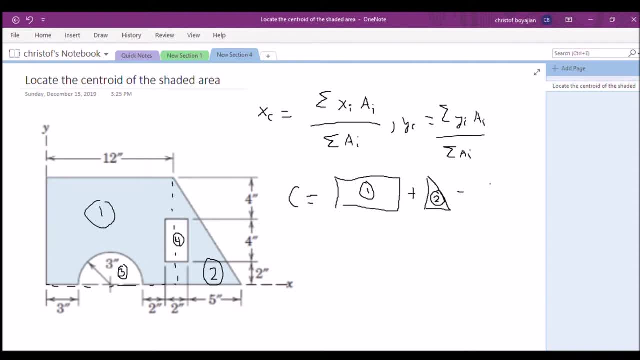 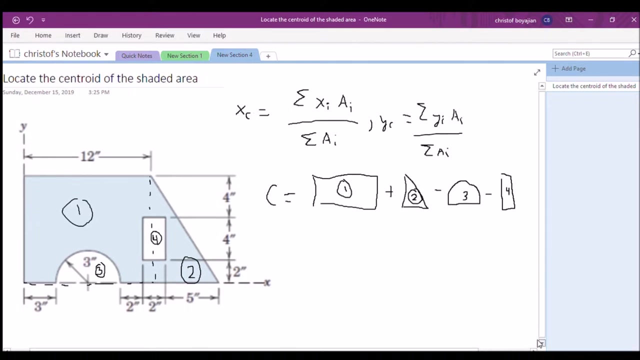 subtracted here. so we're subtracting this semicircle- and i know that's not neat- minus this rectangle right here. okay, so now that we have this stuff, let's go ahead and let's make a table. uh, shall we? now? i'm gonna go ahead and scroll down here. i'm gonna start a table now. this is what i normally like to do. 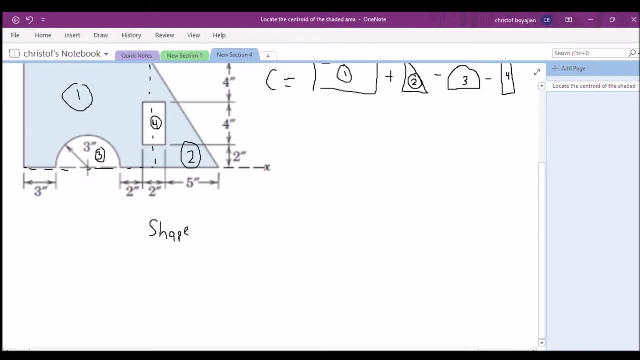 in this table. now i'm going to go ahead and make a table and let's make a table and let's make a table, my tables for the vertical columns. i'll have about like six columns here. i'll write over here. so our first column is just identifying what shape we're going to be dealing with, or we're. 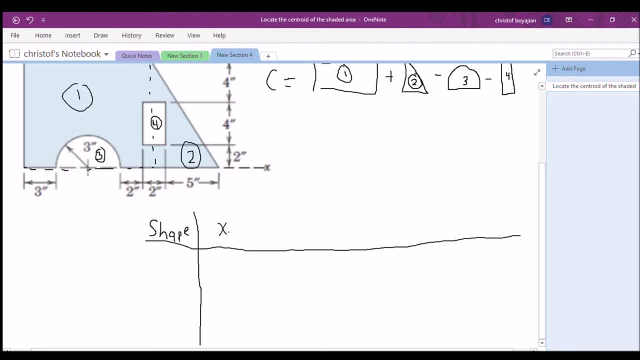 going to be working with, then it's going to be the centroid of that shape in the x direction, then it's going to be the centroid in the y direction, and then it's going to be our total area of that shape, and then, after that, we. the last two things that i'm going to put here are: 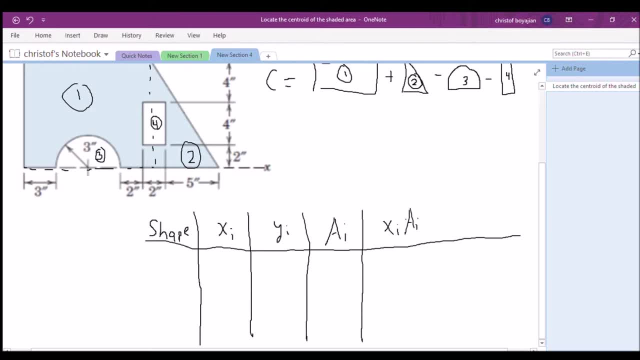 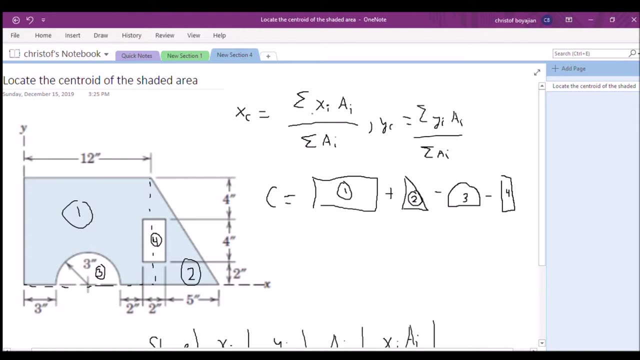 x i a i, and that's just multiplying. this guy right here times this guy. so that's what i'm denoting there, and we need to know what x i times a i is, because by convention or by definition, our form, our formula calls that. and then our y i, you guessed it, our y i times a i. 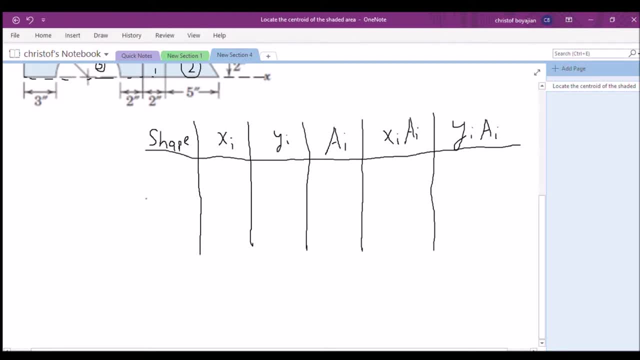 now a i kind of sounds like something you're playing against in a video game, but they're kind of. sometimes the ai can be difficult in a video game. sometimes they can be a little bit easier, depending on how you set the difficulty or depending on how the game works. 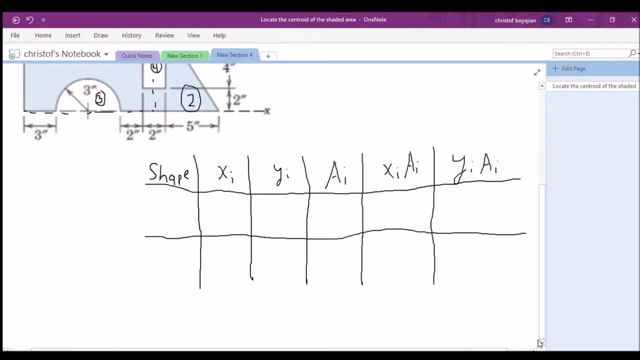 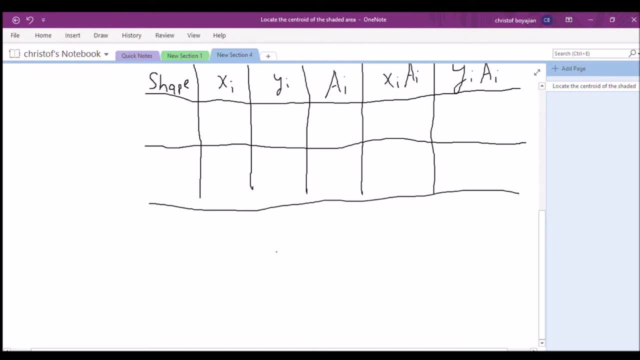 but anyways. so let's go ahead and finish our table. so we're going to have four shapes here, so i should actually make four columns or four rows. so that's three rows. we need one more row. okay, perfect, and let me go ahead and extend these lines down. 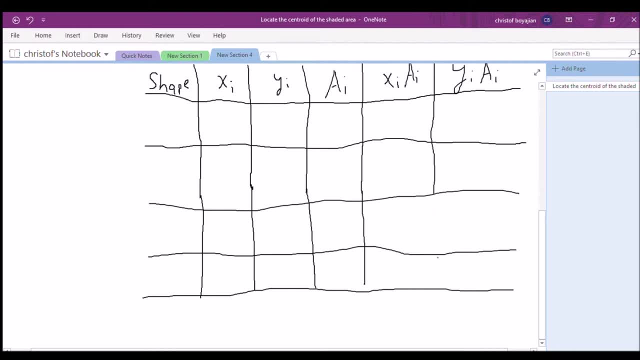 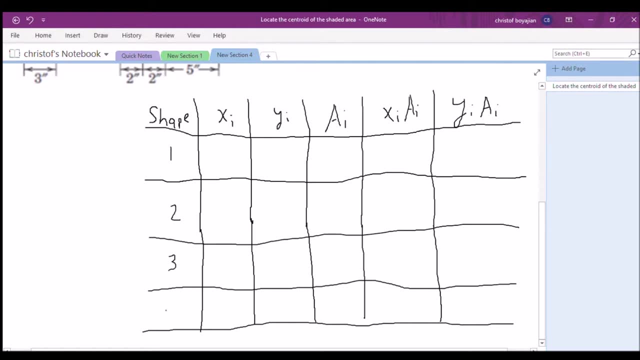 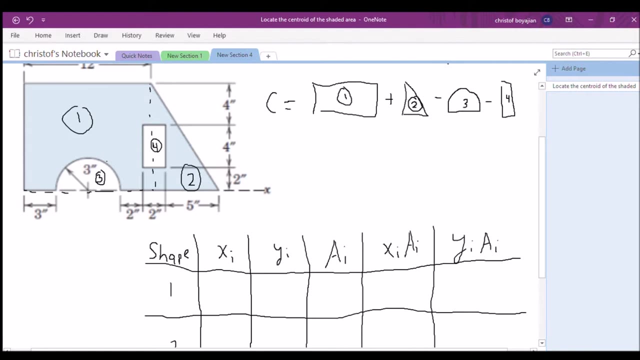 all right, so now let's go ahead and fill out our table. so shape: i'm just going to put one, two, three and four, because we already labeled these shapes. i labeled it as i labeled this rectangle as one. this triangle has two. this semicircular piece is three. 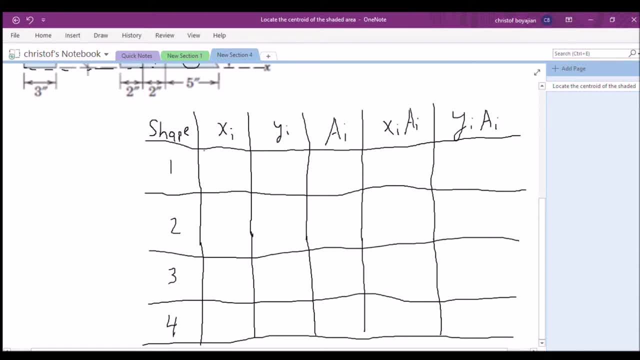 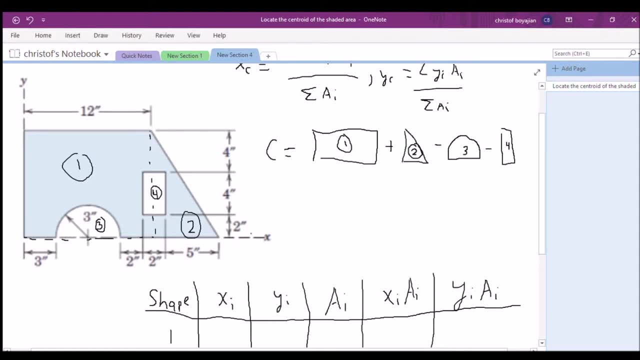 and this, this rectangle, is four. so now let's go ahead and find the centroids of all of these shapes. so remember, when we're finding the centroid of a shape, we want to make sure, uh, we do it with whatever we have the axis uh set to. so we put our origin right over here, so our centroid is going to be a distance from 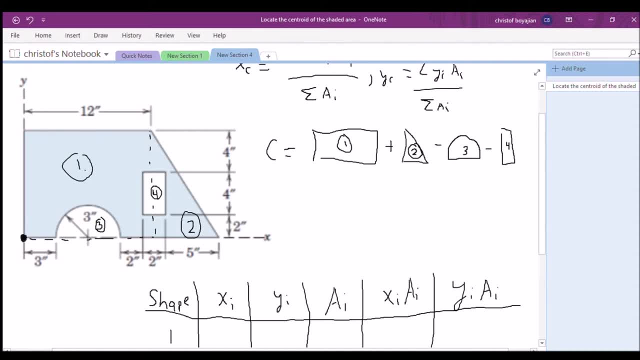 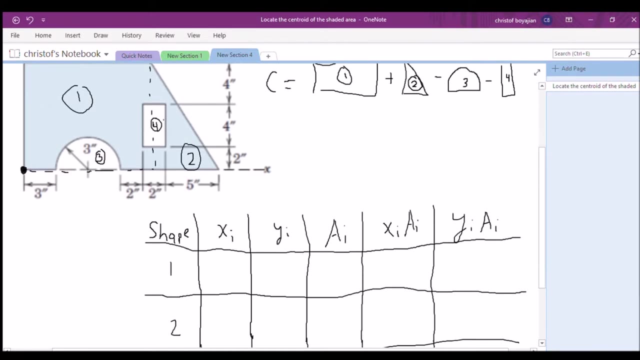 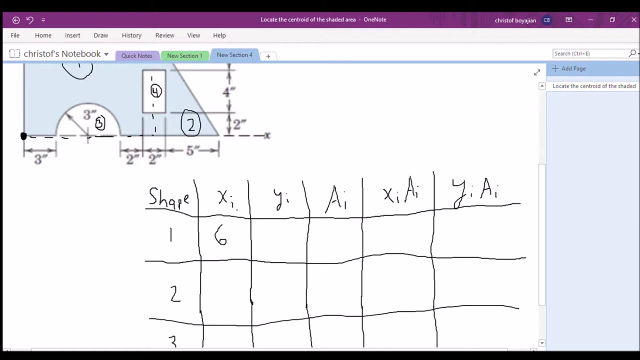 the origin to wherever the centroid of that shape is. so let's start with the rectangle first. now, this rectangle has a length of 12 in the x direction. so over here, our x centroid of this rectangle is going to be six inches. now i'm not going to put the units, because if i were to put the units i'm going to, i would have 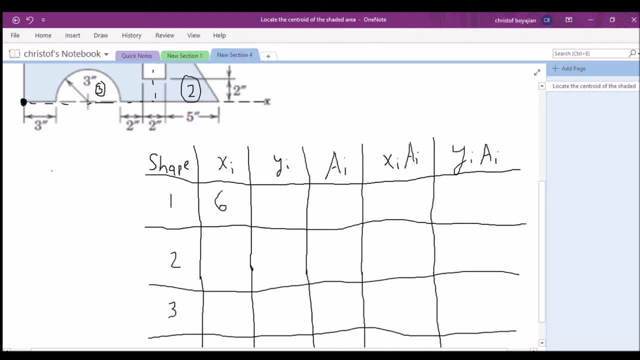 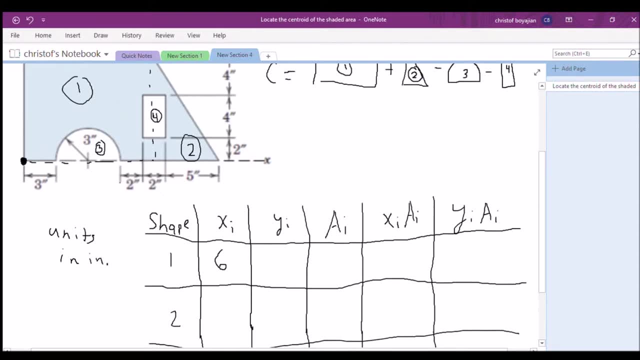 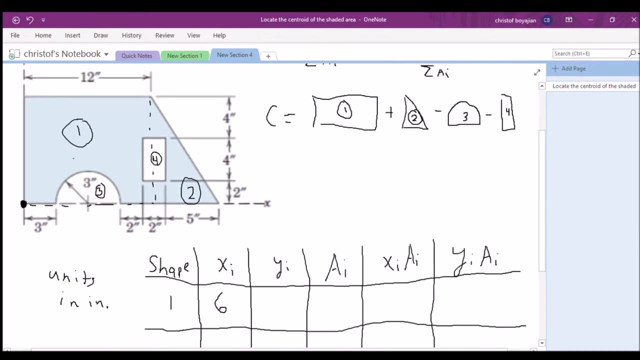 to apply all the units throughout all these columns. so i'm going to say units in inches, right there. units in n, but you know exactly what i'm saying. so, um, that's the centroid in the x direction of this piece. now, in the y direction, it's exactly in the center, uh, of the 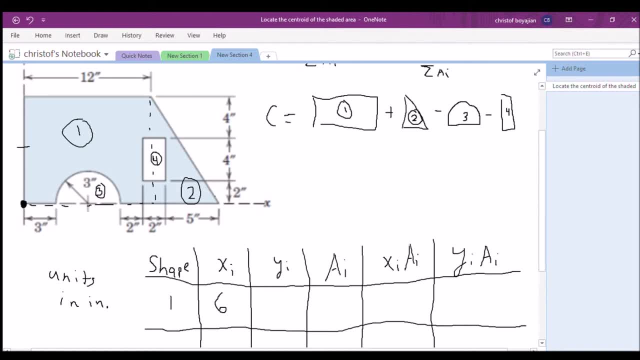 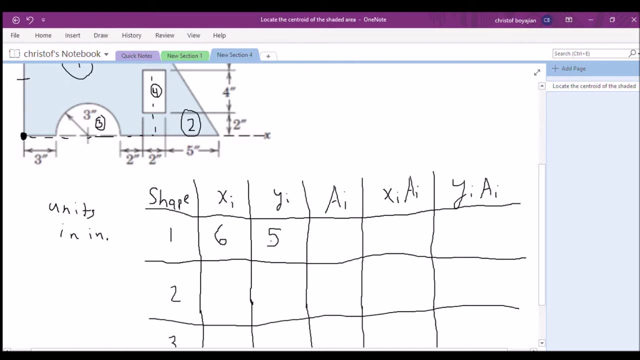 this rectangular piece. so what is this uh length, or this height up in the y direction? well, we have two plus four plus four, which is ten. so our y centroid should be five inches and our total area- let's go ahead and find that, while we're at it now- our total area of this. 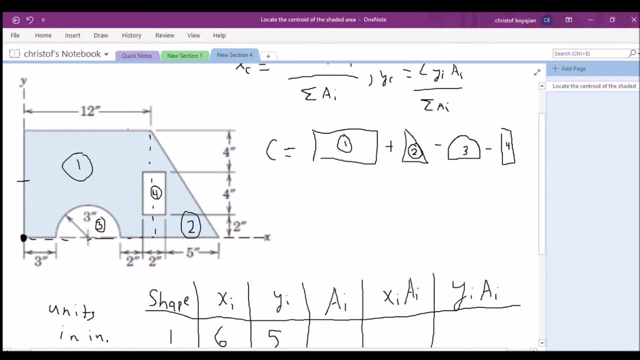 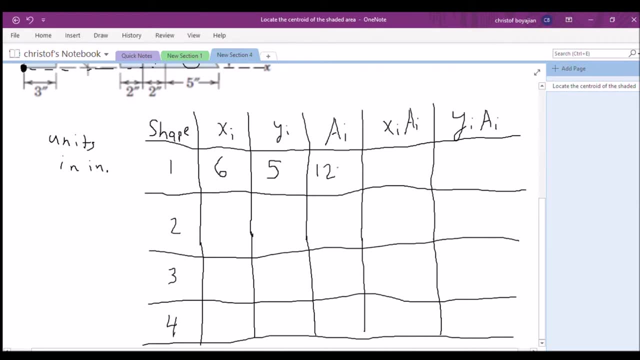 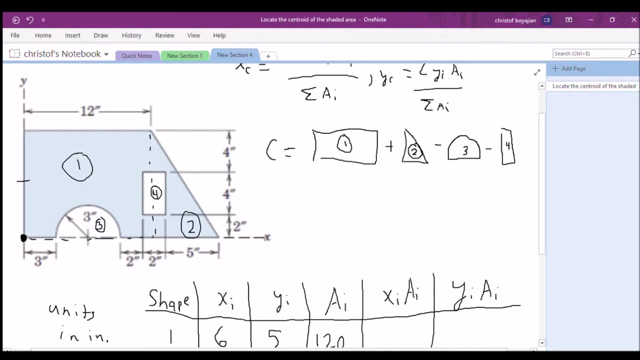 rectangle is going to be, uh, our length times height. that's the area of a rectangle, so it's 12 plus 5 times 10, it should be 120.. all right, now let's go with shape two. so shape two. what is the x coordinate of our centroid over here? so we know from the triangle, or at least from this right. 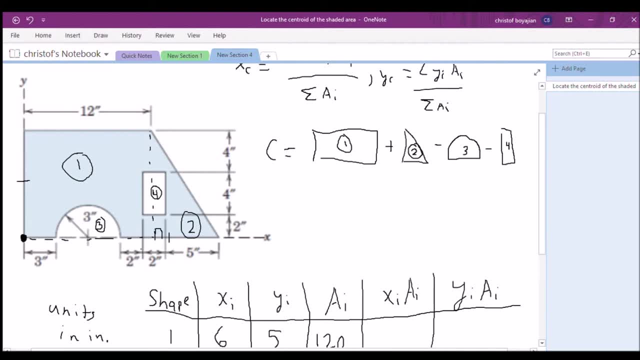 angle. it's going to be one third of that distance to uh, from the triangle right here, at least this distance. we also need to know what this distance is too, because it doesn't give any long distance to where the rectangle is right, and that's how we're going to find that right now. let's 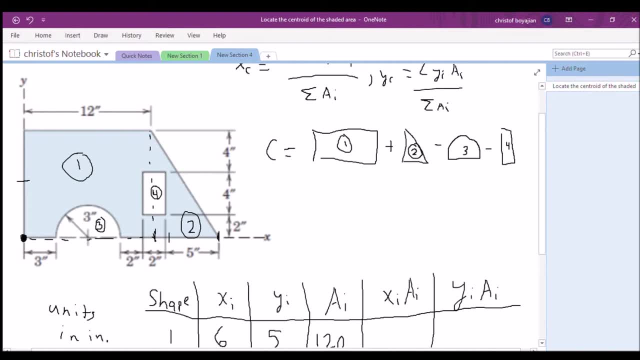 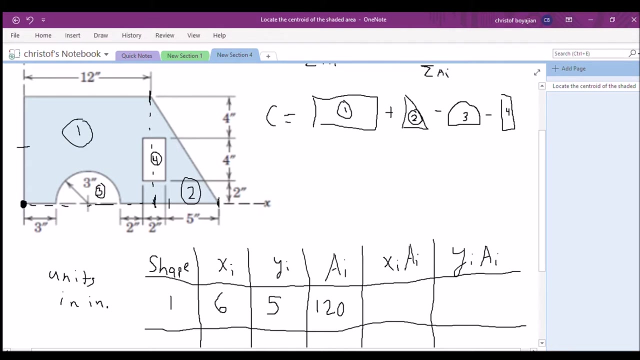 remember, we're adding it from the origin, our distance is from the origin. so what is this distance right here? well, it should be 12, right, because we go distance 12 all the way up to this triangle, and then it is a third of this length of this triangle right here. so what is this length? well, let's go ahead. 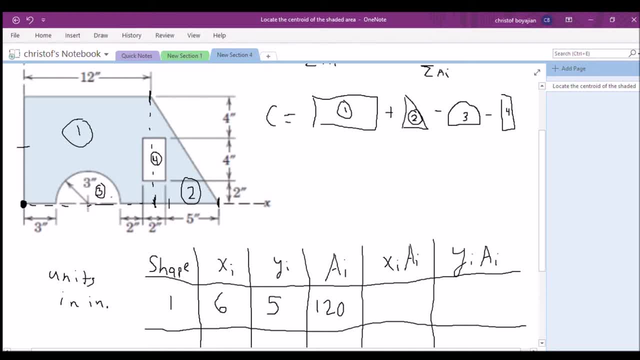 this. this distance is 3, this is 6, because this is the diameter of the circle. so 6 plus 3 is 9, this is 10. so within this 2 right here, this is actually a distance 1 of this little piece right here. so that would make this. 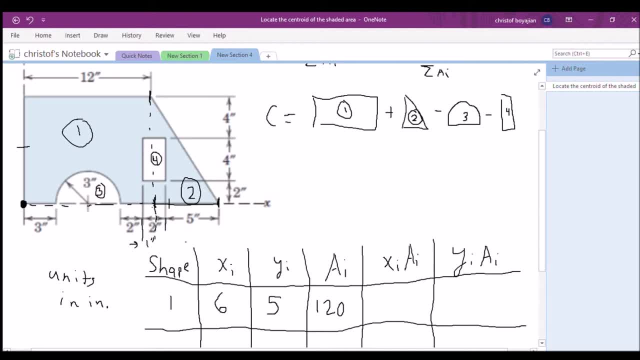 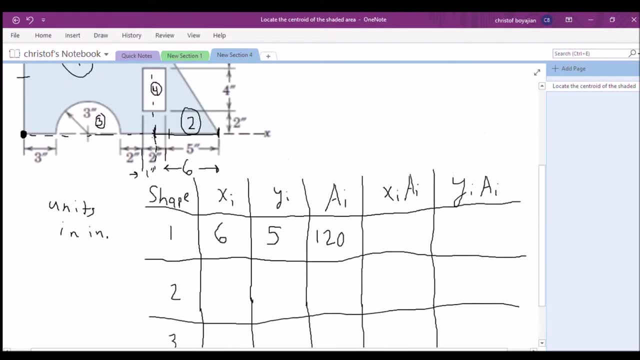 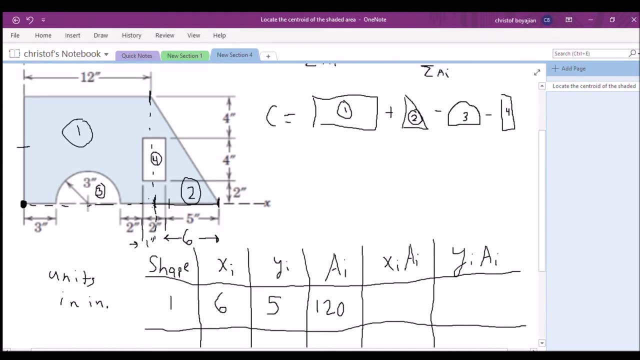 length of this triangle actually 6, right? so 1 3rd of 6 is 2. now we add 2 with the distance that we have over here, so 2 plus the distance to the this leg of the triangle is 14, because we added 12 plus. 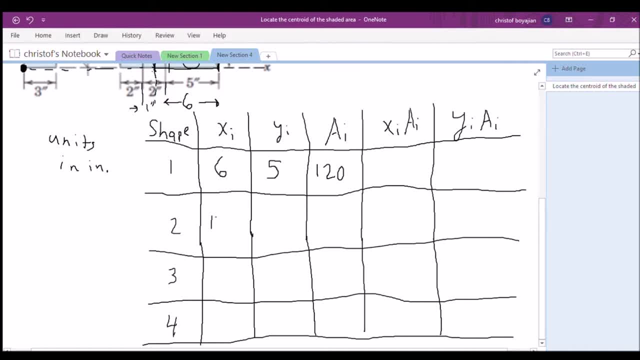 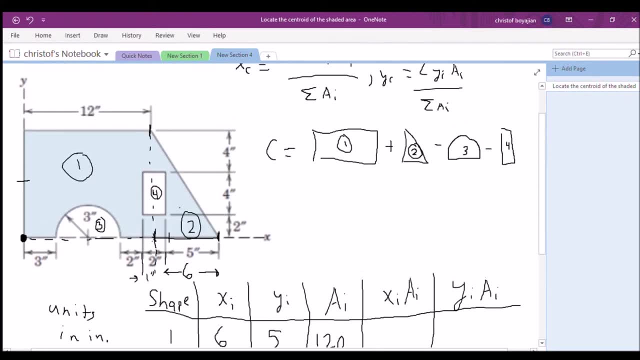 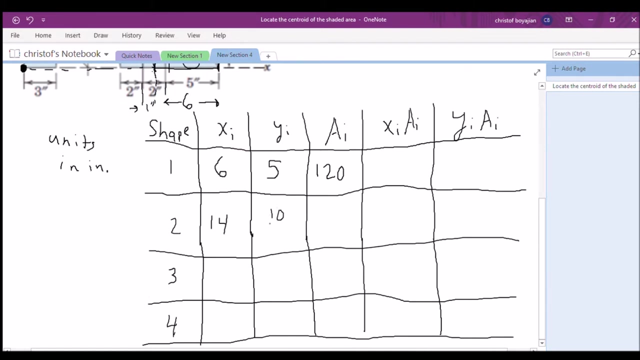 2, so our x direction is 14. now our Y is going to be again 1, 3rd of this distance from this leg. so up, 1, 3rd it's going to be. we see that this is 10, so it's 10 over 3, so that's going to be our Y direction. now our area. what is our? 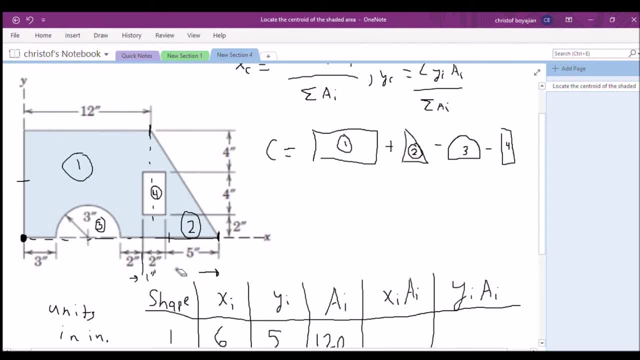 area and let me go ahead and erase some of this. I know it can be a little bit messy. so the area is the length times height divided by 2. that's the area of a triangle. so this bottom base is 6, this top height is 10. so 60 divided by 2 is 30. 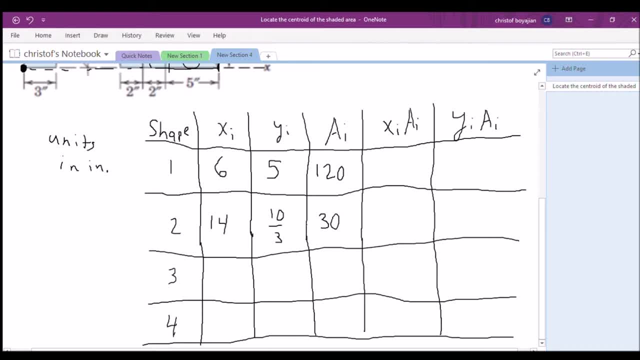 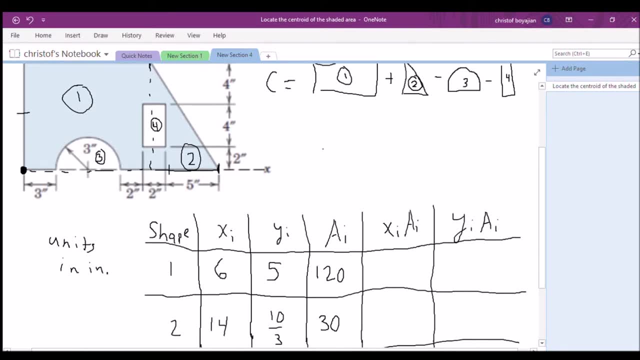 alright, now let's go ahead and do our third shape, which is the semicircular piece. now, remember, for a semicircle, let's say that this is our axis. right, here we put our axis like this: x-axis is along the diameter of the semicircle. the 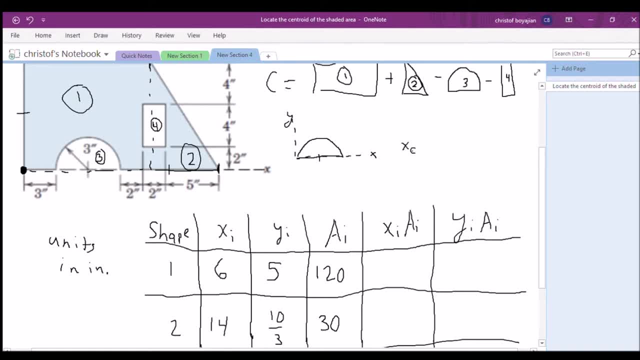 x-coordinate of the centroid is just going to be the radius of that, so I will denote this as R. so we'll say that this is distance R radius. now our Y bar is- or sorry, not our y bar, I'm used to saying y bar- but our y coordinate of the centroid. 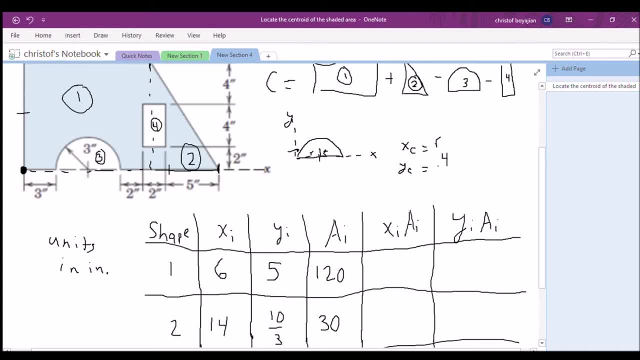 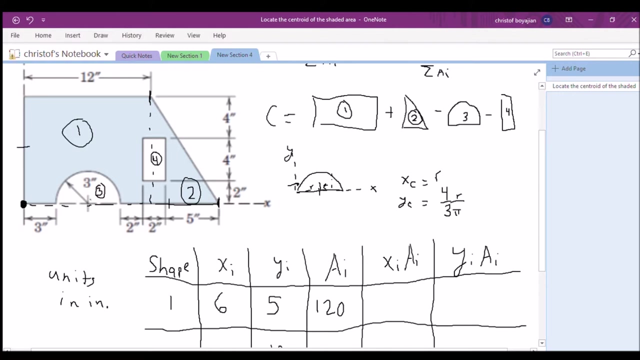 is by using this formula: we use four thirds r divided by pi. Okay, now, that's this distance up from the, from the x axis, up in a vertical direction. So we're going to have to apply that here Now. okay, so, looking at our figure that we have here, what is the x coordinate of the? 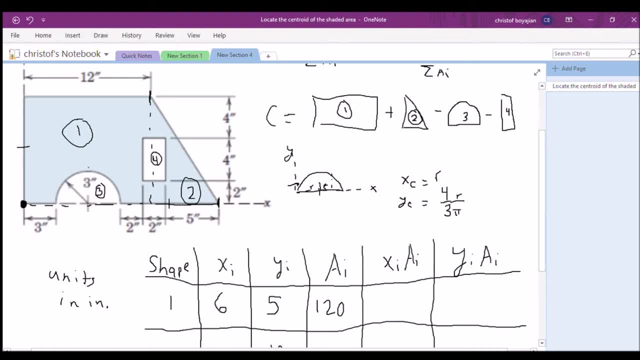 centroid. Well, remember, for the semicircular piece alone, it's a distance r, So this distance is three. this is our radius. it's three, But from the origin what is this distance? all the way over here it's going to be six, six inches. So six inches is our centroid. 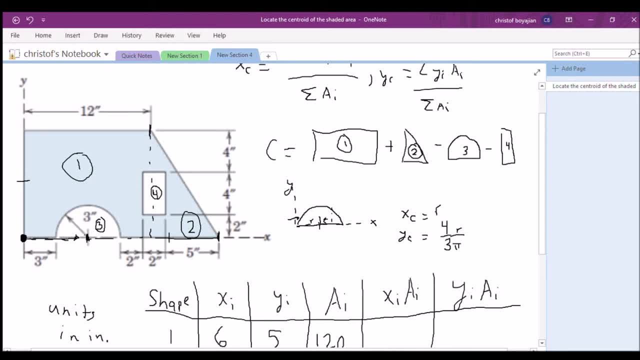 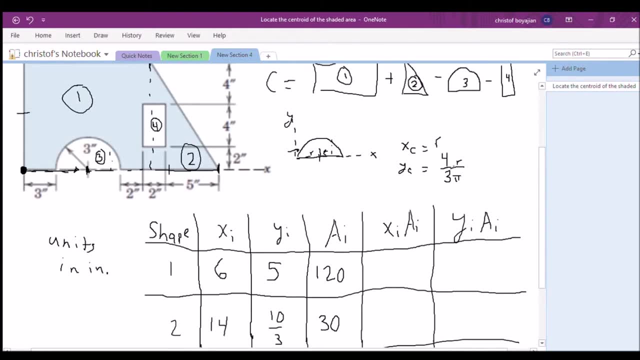 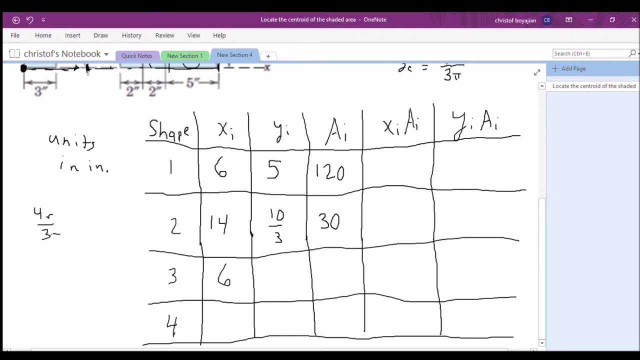 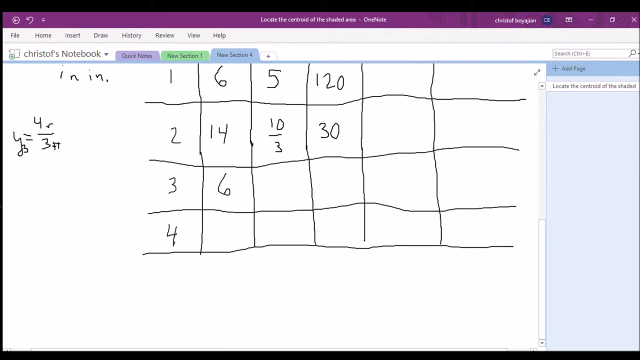 Now our y. now, from the x axis up a vertical, let's use the formula that we have here for r divided by three pi. So for r divided by three pi is our y. I'll put y three, because this is our third shape we're dealing with here. So our radius is three, So four times. 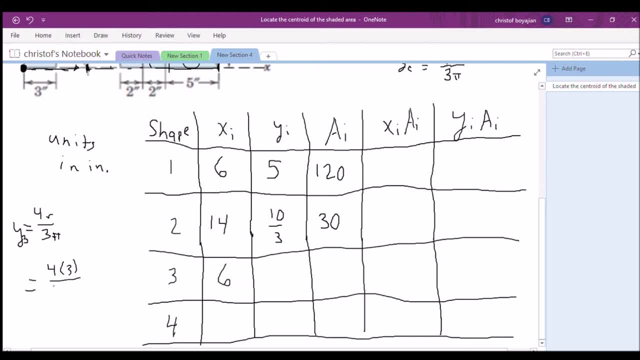 three, Three divided by three pi, And it should just be four over pi. So let's go ahead and put that right here. Or divided by pi, All right Now. our area, the area of a semicircle, is half of that of 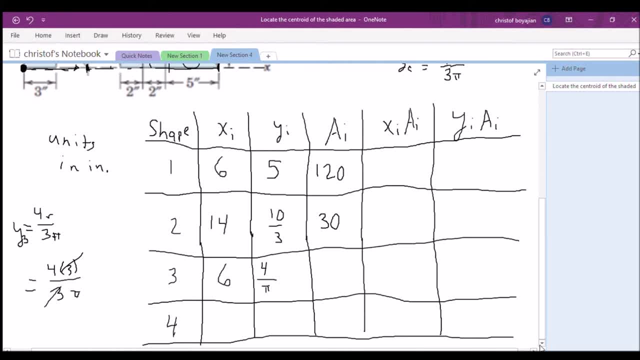 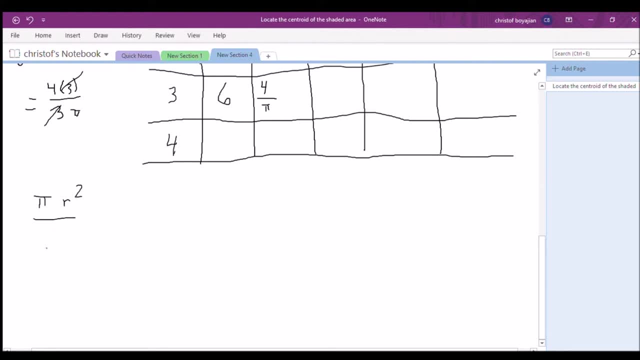 an actual circle. So it's pi r squared divided by two. So the area pi r squared divided by two, our radius is three. So if we go ahead and plug this in, it's going to be nine pi over two, that's. 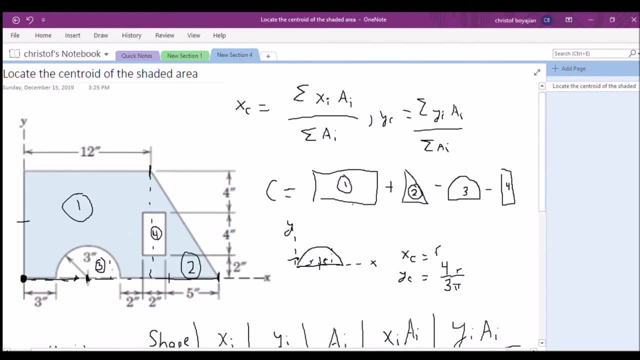 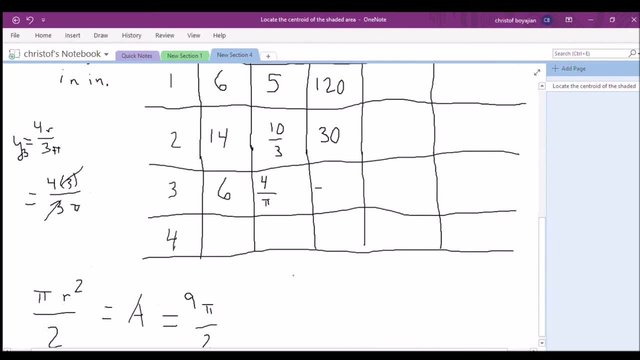 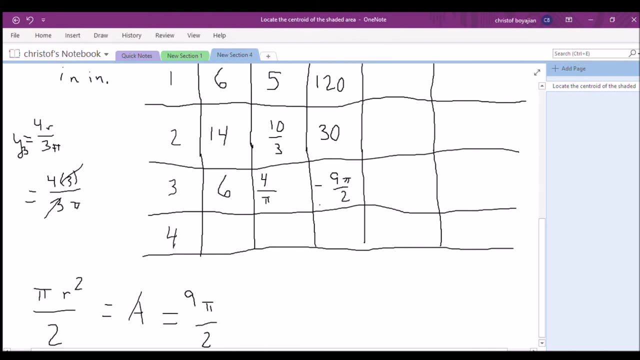 going to be our area. Now, remember, our area is going to be subtracted because this is not shaded in. it's, in fact, open. So this is actually going to be a negative value. Again, I repeat, this is a negative value because this is not a shaded area, So this is actually going to be a negative value. 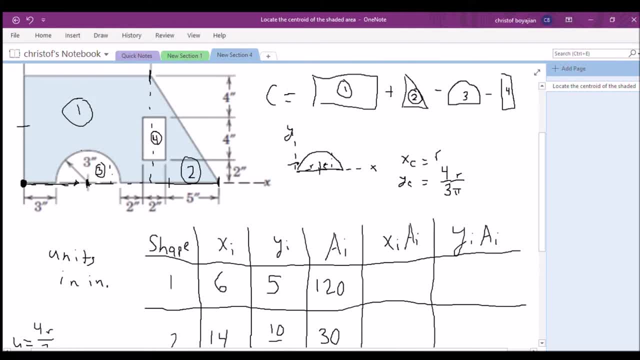 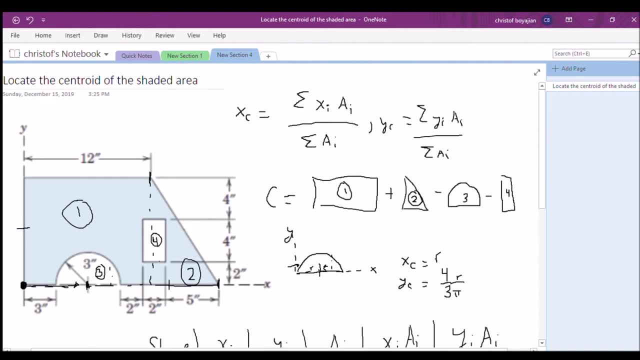 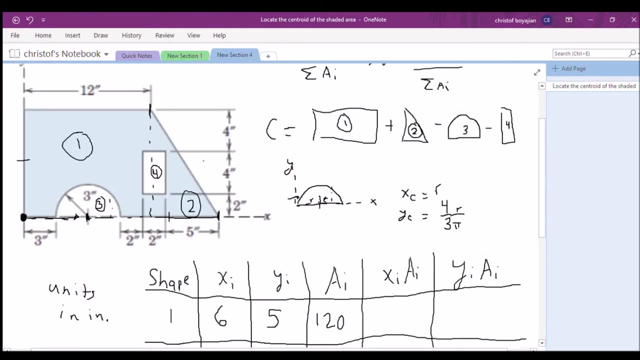 We're subtracting this area to find the centroid, So you can already guess that this area is going to be negative. two, because this is also not shaded. So that's something to keep in mind- is, when you're subtracting areas, you put a negative sign in your little table that you have here. 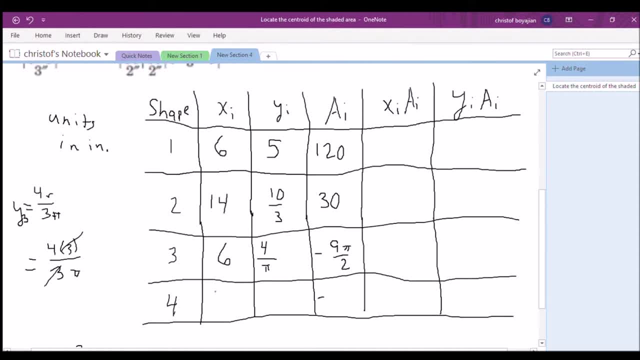 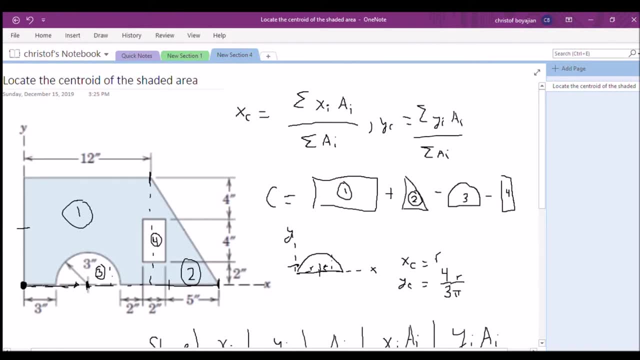 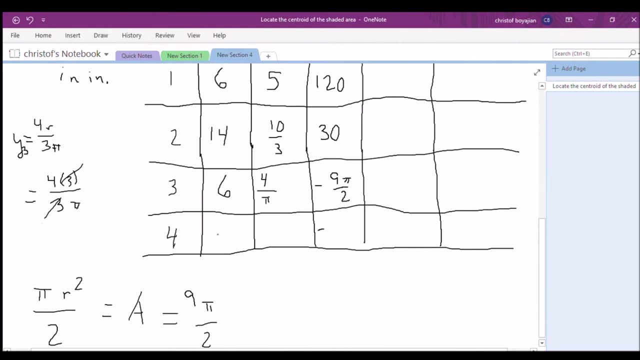 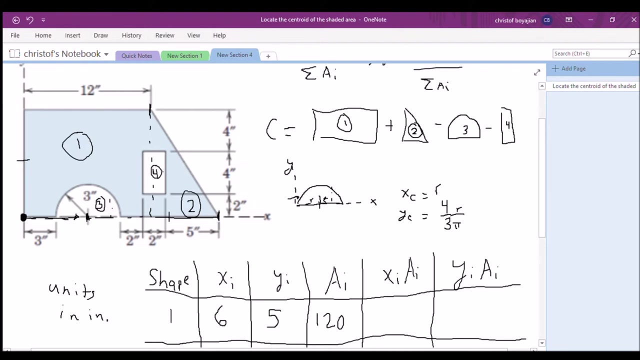 All right. so let's go ahead and solve for the fourth, our fourth centroid And the area. So in the x direction we should have the centroid to being 12 again And our from our y up to here. Now this height is four right, So that means this distance over. 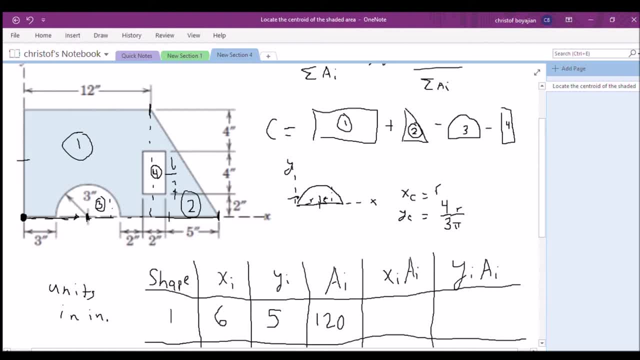 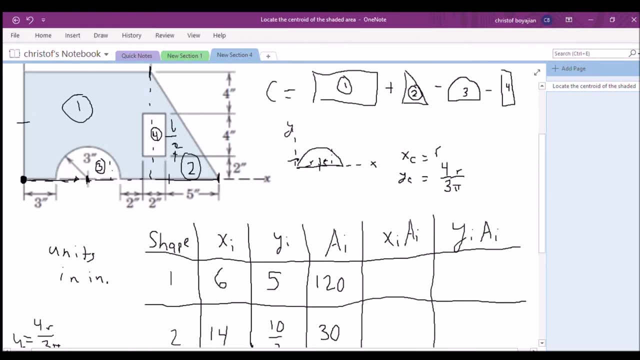 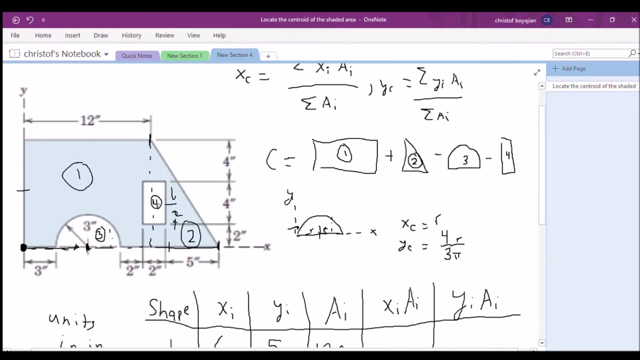 here is two plus two, So that's four. the distance vertically up to here, So that's four. So that means the distance vertically up to the centroid of this rectangle, so it's going to be four. And the area of this rectangle is, so the length of this is to the height of this is four. 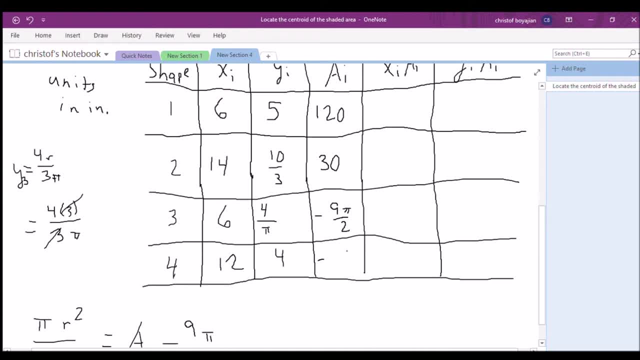 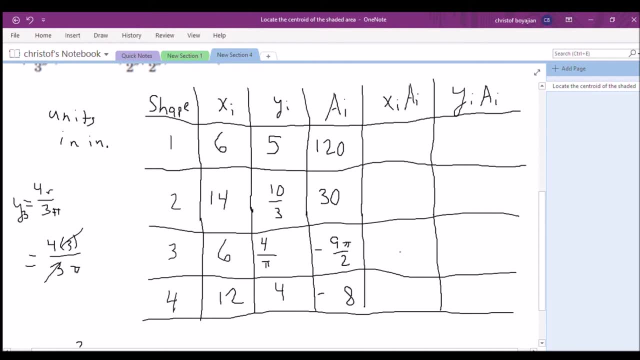 so the total area is eight and it's negative. so we already put that All right, Now that we have done the meat of our work here. now all we have to do to fill out for our x i times a i in our y i times a i is just simply. multiplying. By doing a simple multiplication, we can multiply our y i times a? i into four, and that's what we're going to do Now. all we have to do to fill out for our x i times a? i and our y i times a i is just simply multiplying. 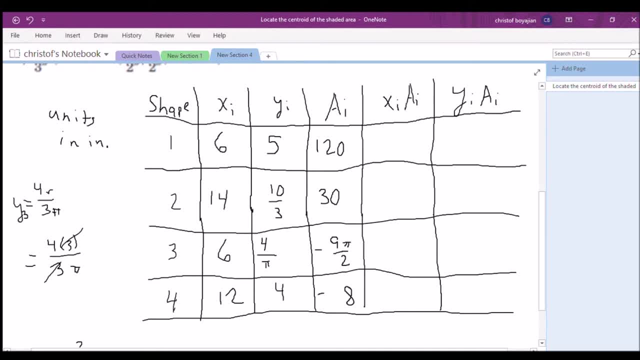 So we multiply 6 times 120 to get XIAI for our first shape. So if we do that, 6 times 120 is 720.. And then 5 times 120 should be 600.. Okay, now let's go to the second shape. 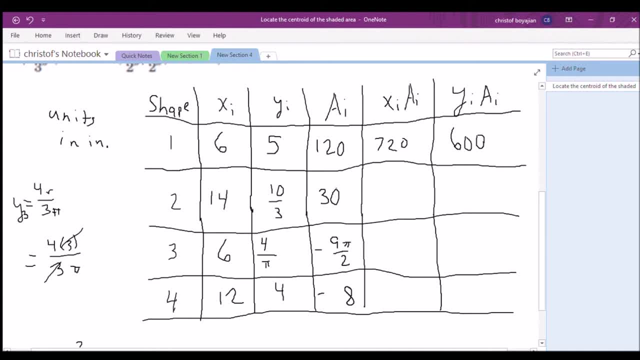 14 times 30 is 420, right, Yeah, 420.. And 10 over 3 times 30 is 100.. Well, not 1,000, 100.. Okay, Okay, Now when we multiply our third and fourth areas, together with our centroids. 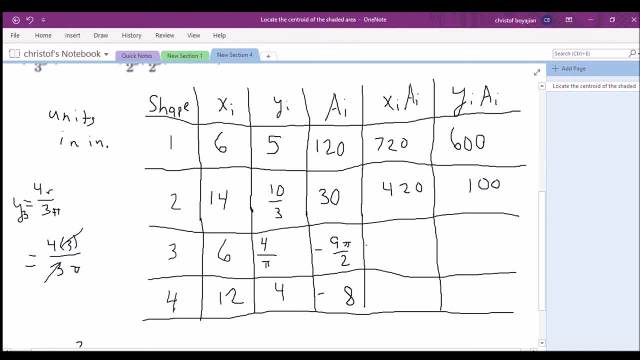 we have to multiply with the negatives too. So when we multiply, When we multiply with our negatives, these are actually going to be negative too, And I'm just going to go ahead and write them out at the beginning, so that way we don't forget about multiplying the negative. 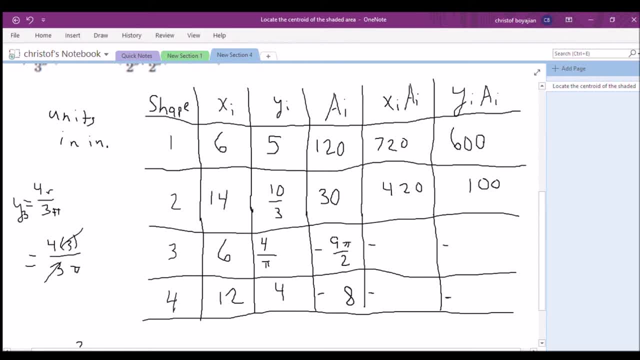 because it's oftentimes easy to forget about the little negative there. So we need to keep that in mind. So let's go ahead and do that. So 6 times 9 pi over 2, that's going to be 27 pi negative. 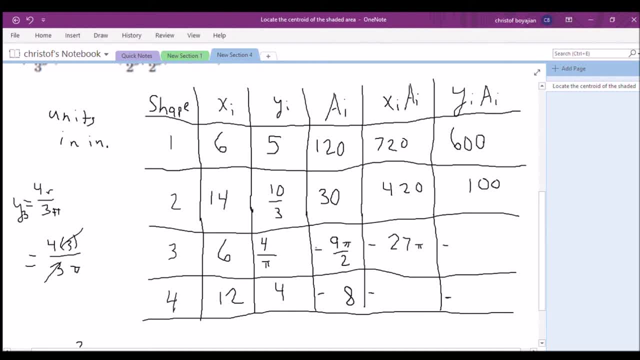 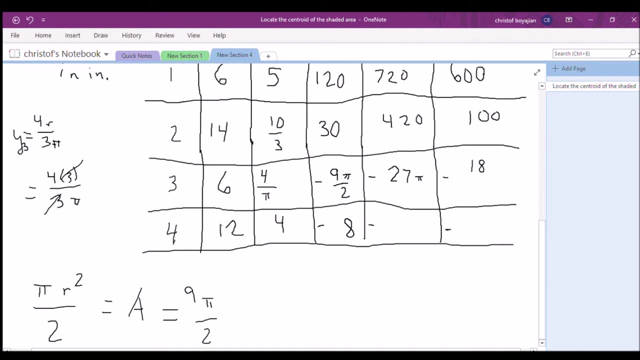 Now 4 over pi times negative, 9, pi over 2.. So pi's cancel out. We got a 2 on the top, so it's negative 18,. I think, Yeah, negative 18.. And then on the bottom we have 12 times negative 8, which is negative 96.. 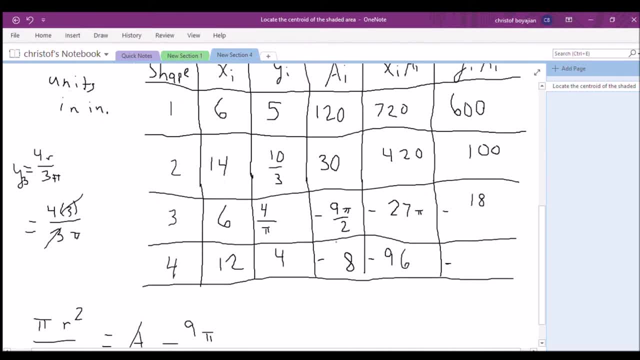 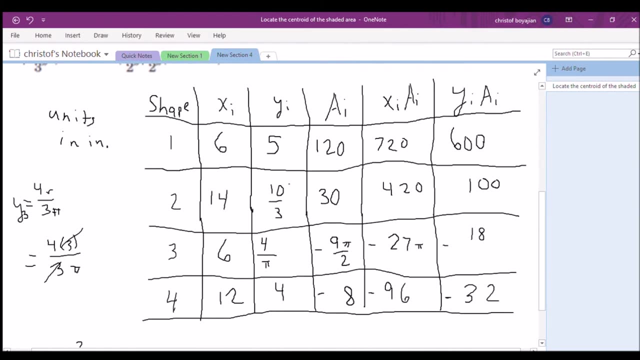 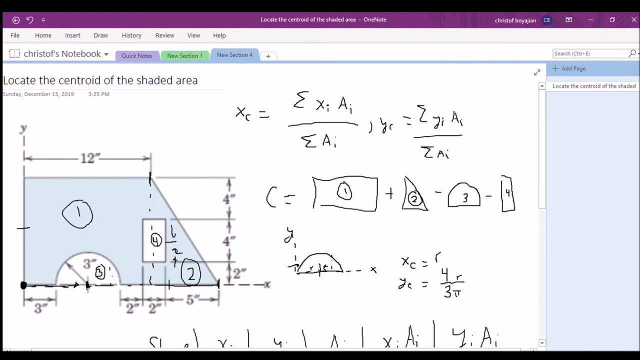 And for yi times ai, 4 times negative 8, we get negative 32.. All right, so we have now completed our table. Now, the next thing that I'm going to do is, for our formula, we need to know the sum of all of the xi ai's, yi ai's and the sum of all the ai's. 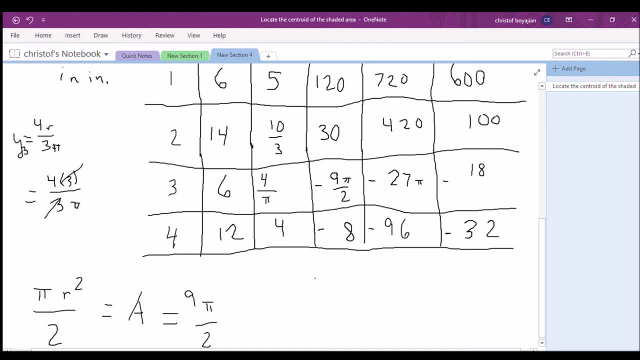 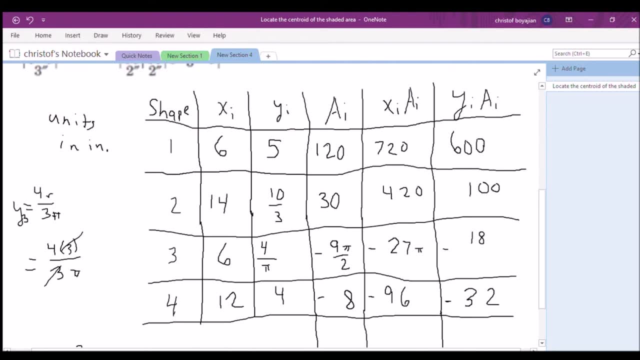 So let's go ahead and sum all of these three components right here. So I'm going to go ahead and do that And to sum, it's just basic addition. So if I go ahead and plug this into my calculator, so 9 pi divided by 2, and that's negative. 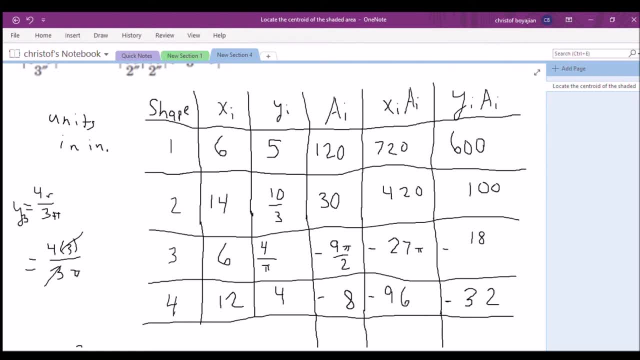 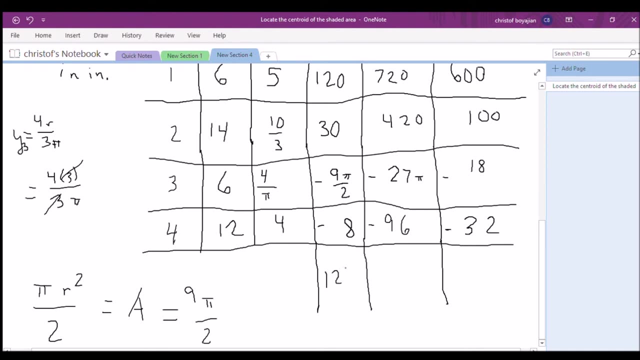 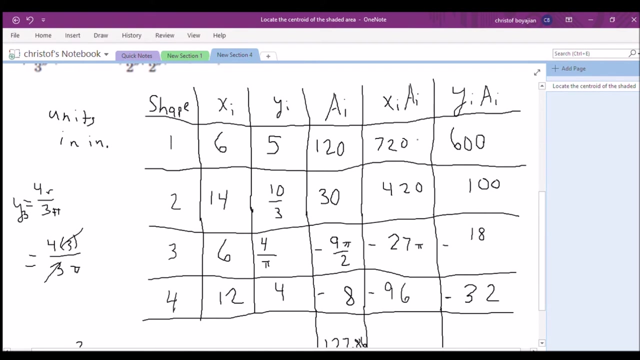 So let's go ahead and multiply that by negative 1, plus 30, plus 120 minus 8.. So this total area is 127.. And then I'm going to go ahead and do this. So 720 plus 420 minus 27, pi minus 96 should be 959.17. 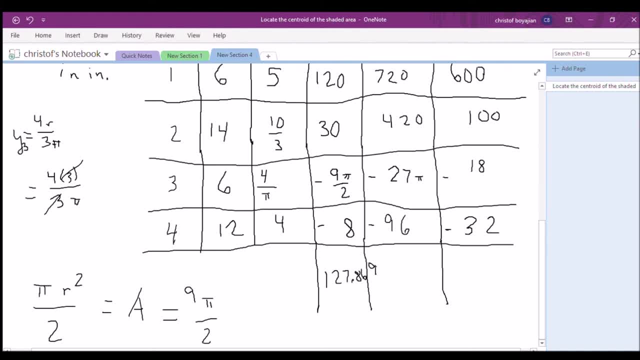 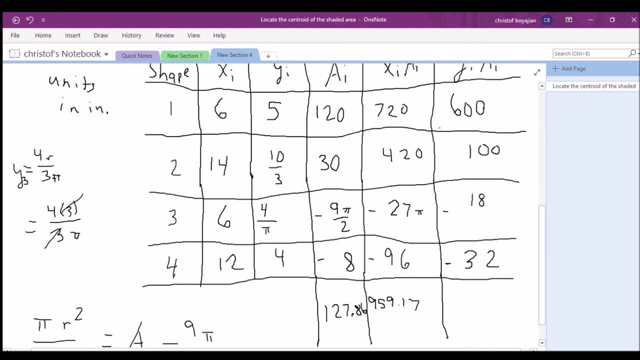 So let's go ahead and write that 959.17.. And this is 600 plus 100.. Minus 18, minus 32, 600, forgot to carry that over 600, minus 18, minus 32.. 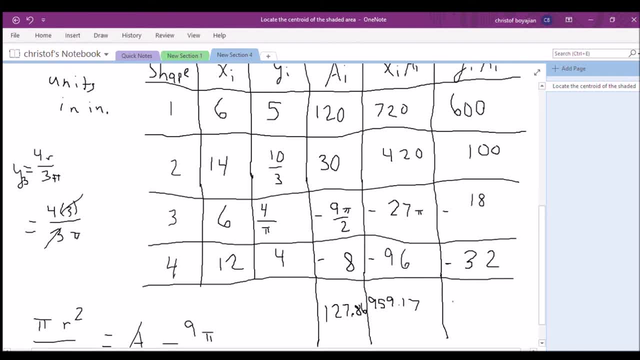 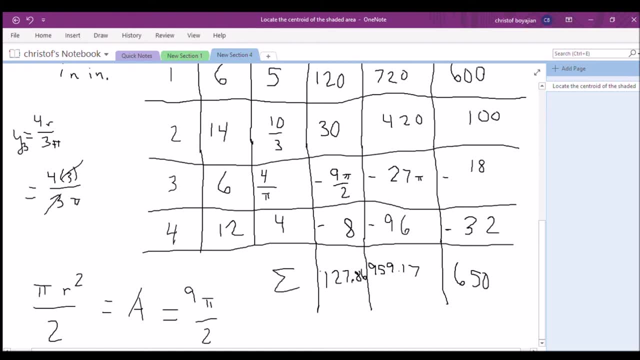 And we got a grand of 650 over here. Now, remember, this is us doing the summation of all of these, So I'm going to put a sigma right here to denote that this is what we're summing up here, And so, now that we have finished, 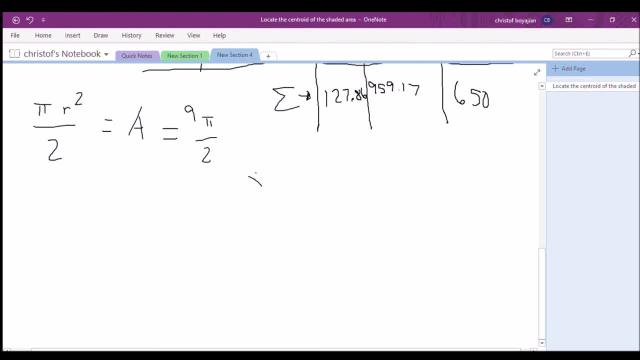 completing, summing up all of those terms, let's go ahead and solve for our x-coordinate centroid and our y-coordinate centroid. So we have. I'll rewrite the formula right here again, Again, to recap, it is the xi times ai sum divided by the sum of the ai's. 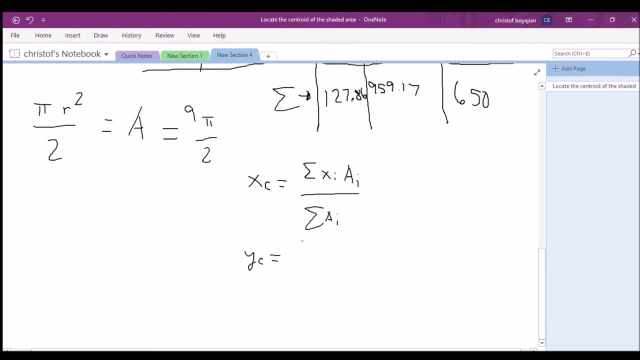 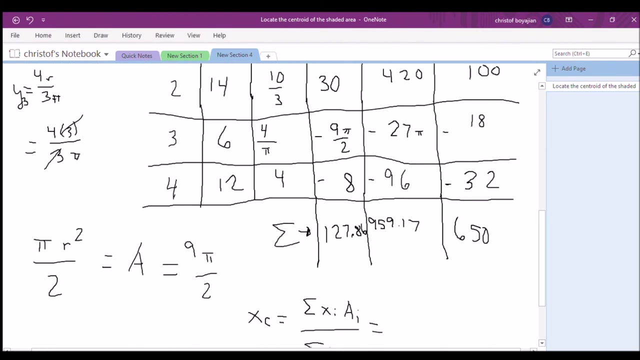 And our y-coordinate is the same thing, except it's just our yi times ai sum divided by the ai sum. Ooh, Sigma, Okay, So now let's go ahead and plug and check. So xi ai sum is- let's see, it is 959.17.. 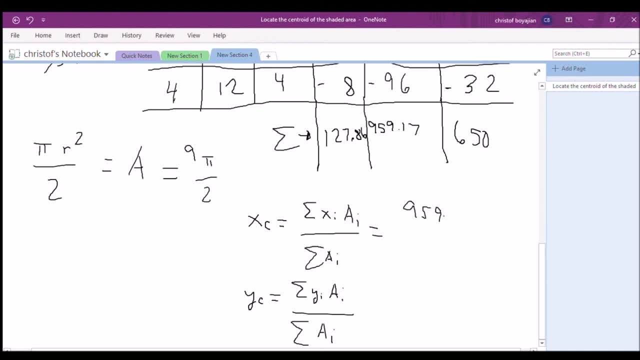 We look down at the vertical column 959.17.. And our total area, the sum of all of our areas, is 127.86.. This is a 7.. And then for our yi ai. our yi ai sum is 650 down here. 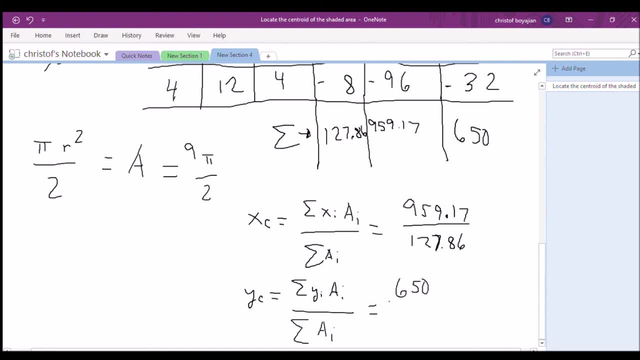 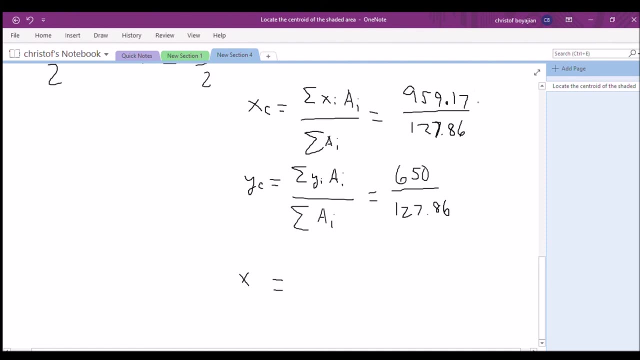 After we concluded, our sums divided by our total area again, it is 127.86.. Now let's go ahead and solve for the x-coordinate of the centroid and the y-coordinate. Actually, I might have room to write it here. 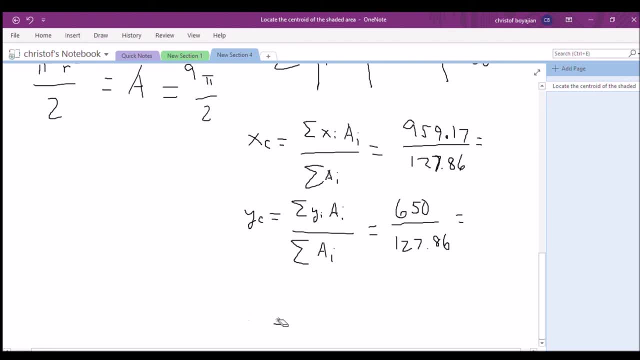 So I'll plug this in the calculator really quick And see what we get. And we should get. so: 959.17 divided by 127.86.. It is 7.50.. Okay, I'll leave it at 7.50 inches. 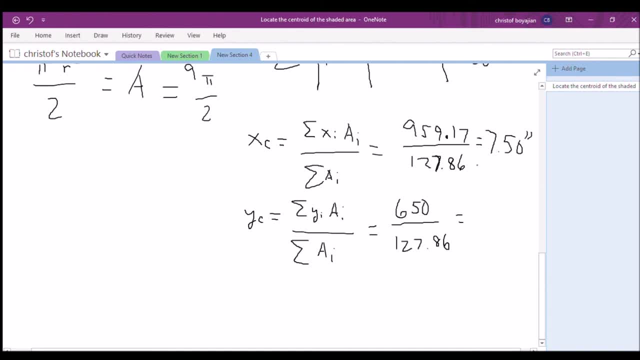 And our y-coordinate is 650 divided by 127.86.. And that gives us 5.08 inches, 5.08.. Draw a better 8.. There we go, All right, So there we go. That is the centroid. 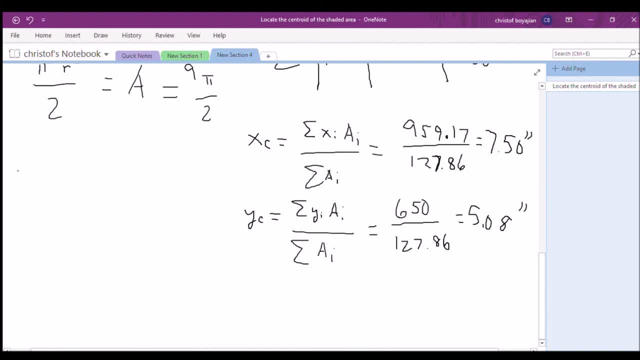 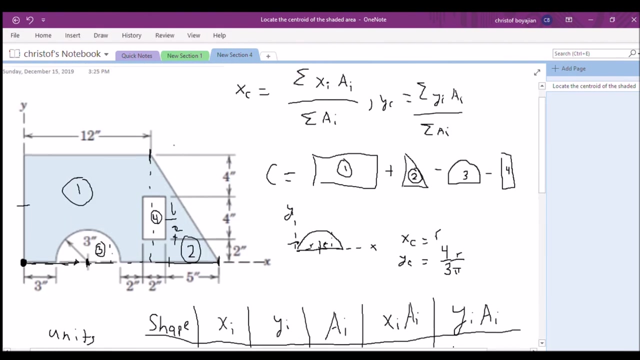 And I'll go ahead and rewrite this here. So our coordinates of the centroid is 7.50. Comma, 5.08 inches. So this is our solution: set of this monster. All right, Hope you learned something today And I hope to see you in another video. 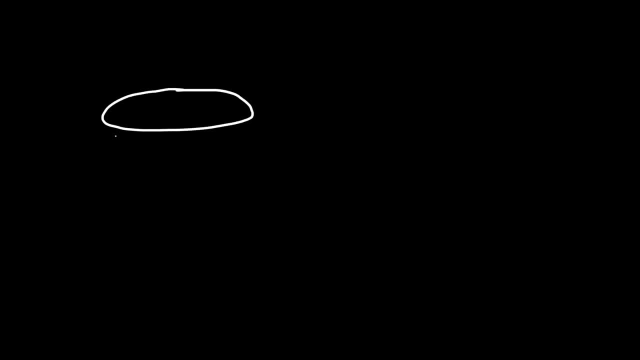 In this lesson we're going to talk about how to calculate the volume of a cylinder. So let's say the radius of the cylinder is 5 inches and the height of the cylinder let's say it's 10 inches. So, using this information, what is the volume of the? 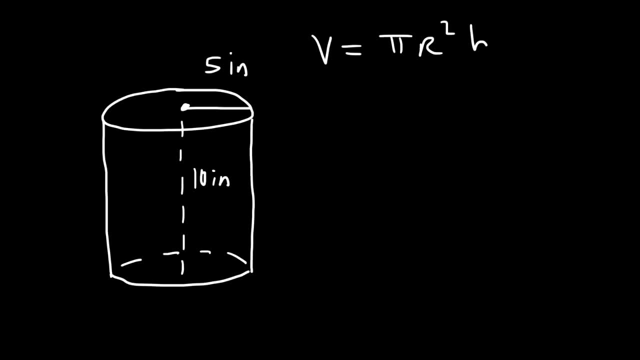 cylinder, The volume is pi r squared times height. It's basically the area of the base times the height of the cylinder. So for any prism the volume is base times height, The area of the base, which is the area of a circle, that's pi r squared. 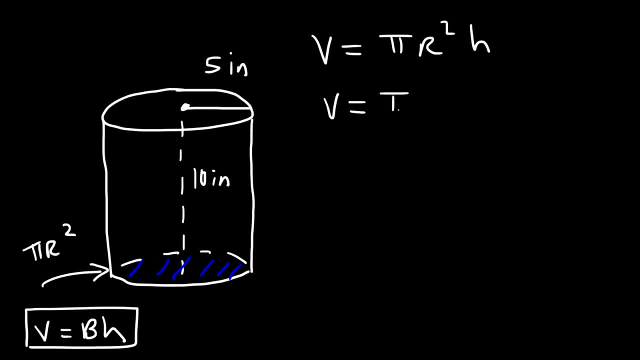 and so it's pi r squared times h. In this example, the radius is 5, and the height is 10.. 5 squared is 25, and 25 times 10 is 2,000.. So the volume for this cylinder is 250 pi and it's cubic inches. 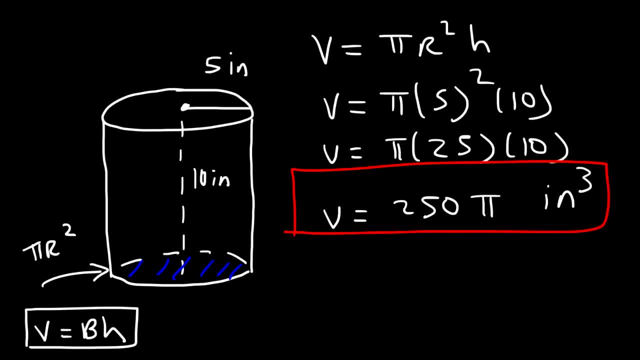 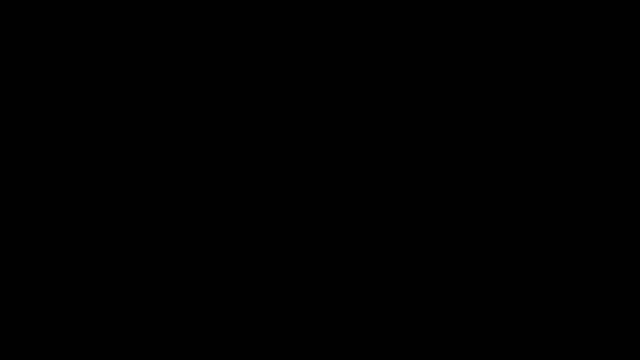 So that is the answer. Now, if you want to get the decimal value of that answer, it's approximately 785.4 cubic inches, And there it is for the radius of theensemble. This is what the value of the original value is. 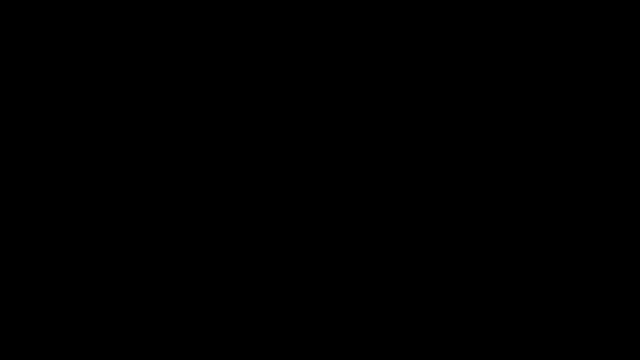 And then I'm going to talk about some other questions that are still there. So this was, but this was like all of Northeastern science at its final stage of development, But anyway, it's an interesting way to look at it, Right.